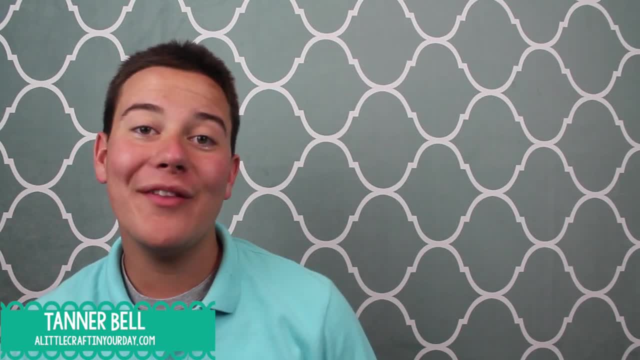 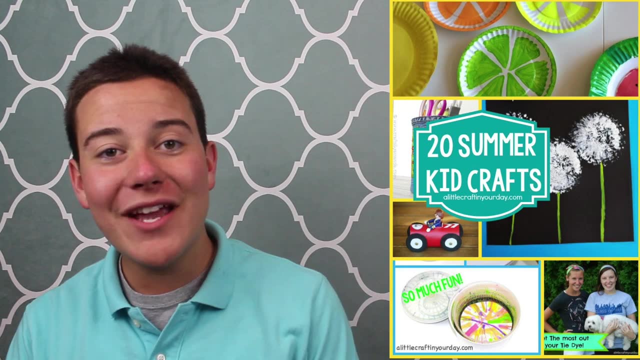 Hey everyone, welcome to LittleCraftsYourDaycom. My name is Tanner Bell, the Editor-in-Chief, and in today's DIY tutorial, we're sharing 20 summer kid crafts. You're gonna love this video, so let's get started. 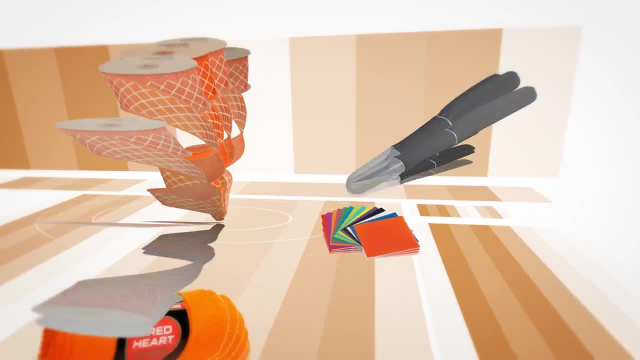 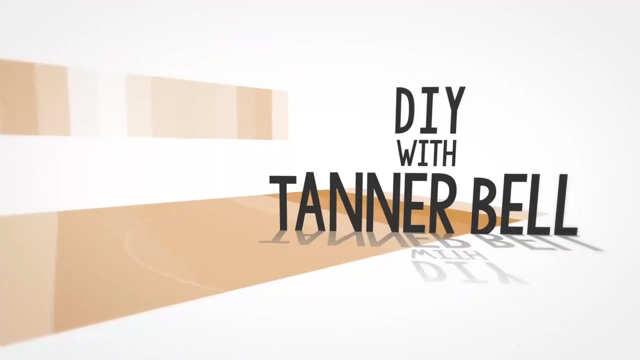 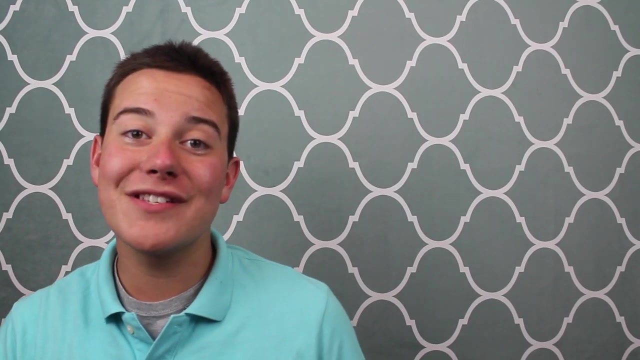 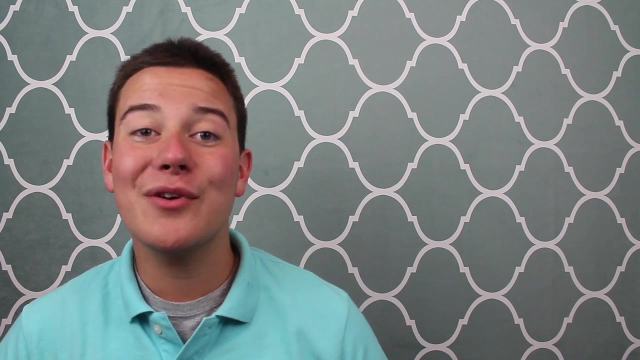 I know you guys have been looking for tons of summer kid crafts to do with your kids this summer and it's the dog days of July and you are going to be needing these. So I'm going to share 10 of them in today's video and you can click on the link in the 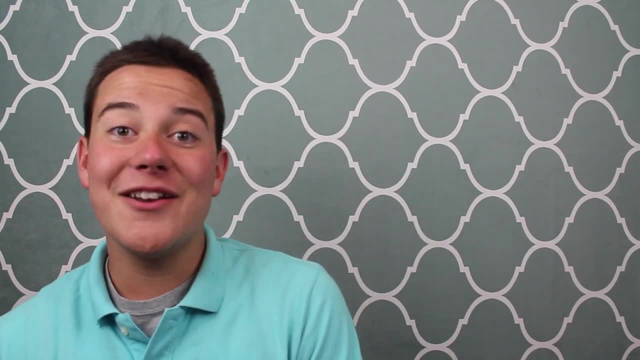 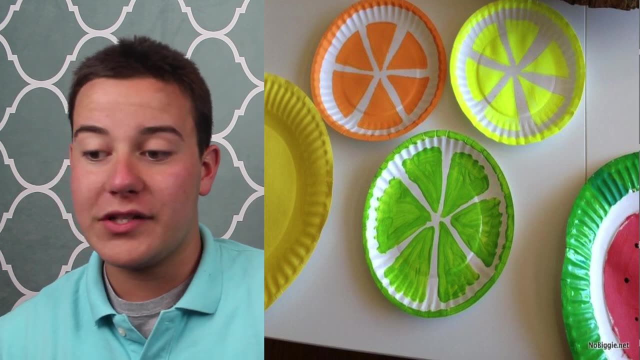 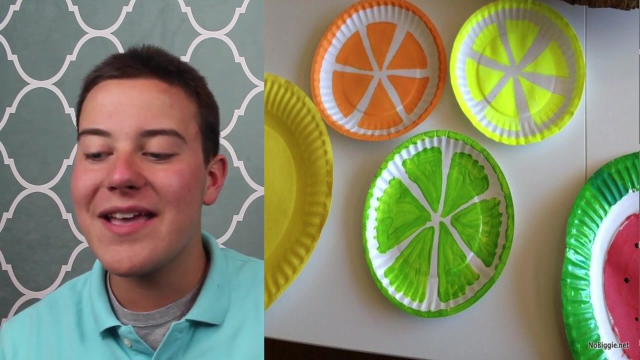 description below to check out the other 10.. These are awesome ideas and I know you guys will love them, So let's get started. Number one is the paper plate fruit. This is a really fun one, and the kids can take paper plates which cost about a dollar for about 50, and they can paint on it and they 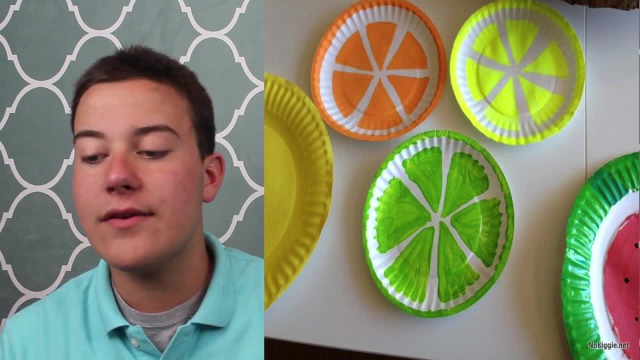 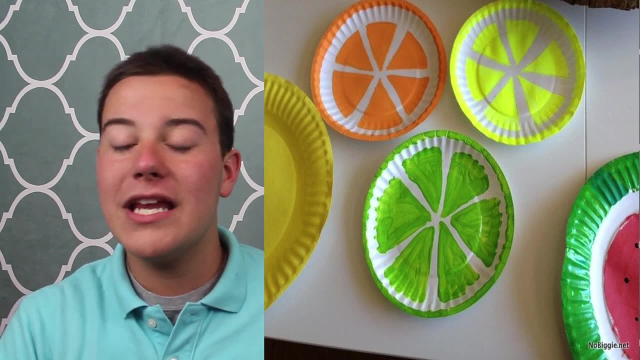 don't even have to do fruit. They can just paint on them or do anything you want. Now I would do draw a watermelon on mine because I love watermelon and literally obsessed with eating it. but that's just me, And I remember I do have some watermelon in the fridge, so I'm going to eat that after. 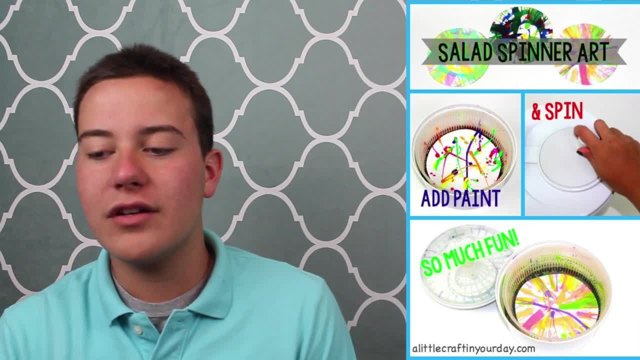 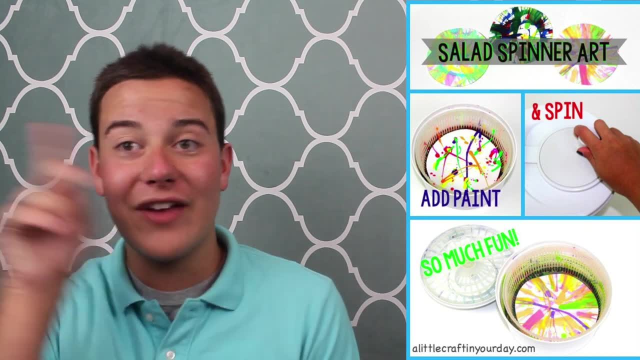 I film this. Number two is one that Courtney over at Little Craft Junior Day created, which is salad spinner art. We did that when she was babysitting one day while I was up in Pennsylvania when I filmed two other episodes of the show, but I'm home now in my regular set, So it's a. 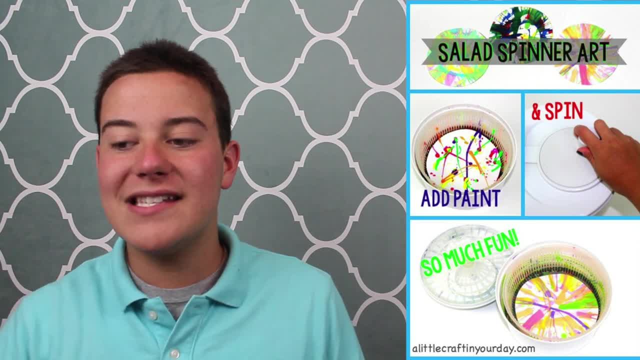 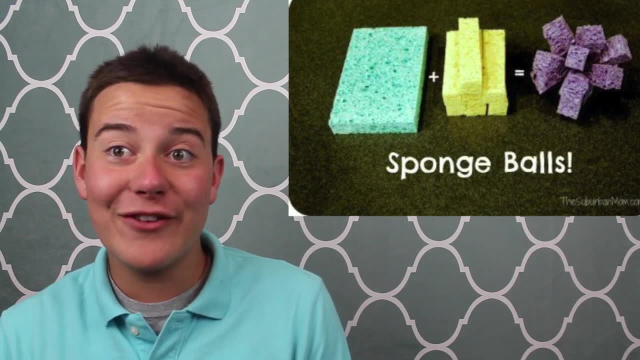 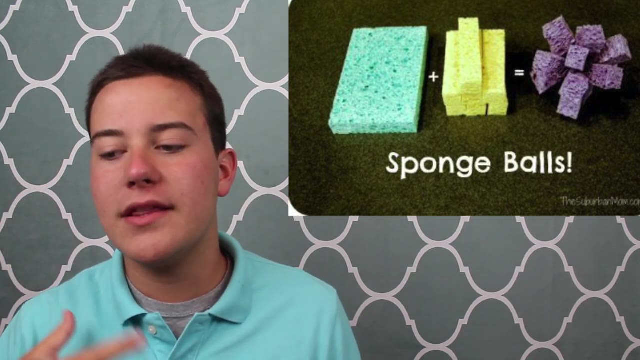 really fun idea and it's super easy if you have a salad spinner, which is a really neat thing to have. Number three is the sponge balls, and these are so much fun, especially for the pool, when you're having a water sponge fight, which would be sort of like a water balloon. but 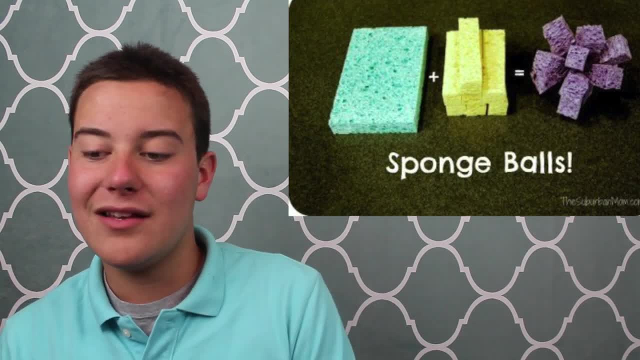 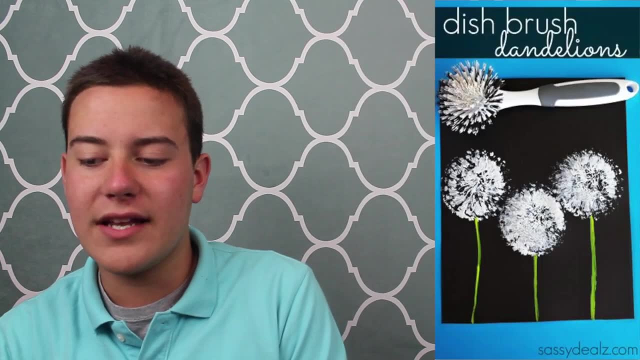 these are easier and they don't pop, So it's really neat and the water just hits the person, which is pretty cool. Number four is the dish brush daffodils or dandelions. Dish brush dandelions- Sorry. 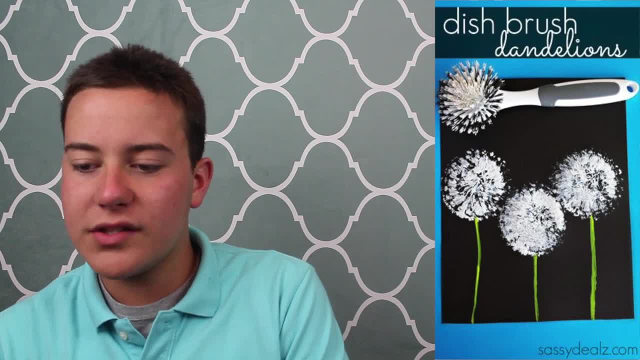 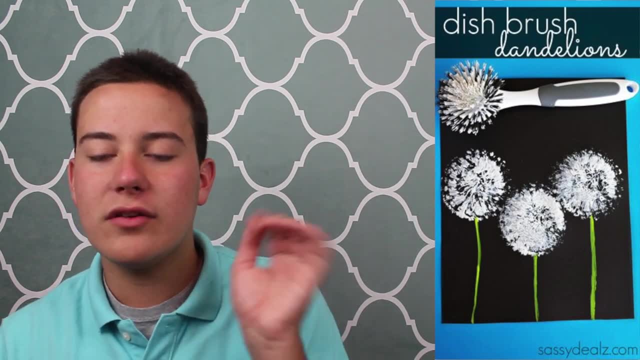 about that. This is an unbelievably cool stamp. I used to love to stamp. I used to use different materials as stamps, so this one's really fun and you can just use regular acrylic paint to be the ink for the stamp. so it's really cool and you can. 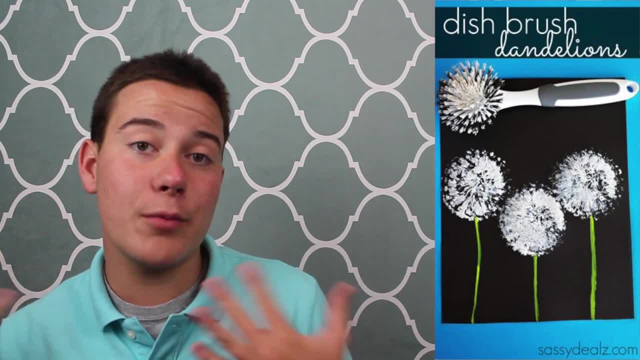 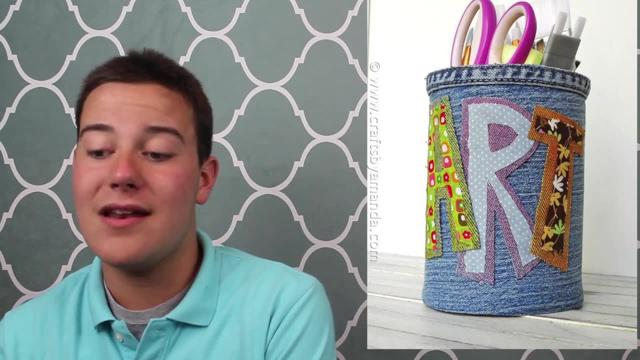 pick up a bottle of acrylic paint for 50 cents to a dollar per bottle. That's pretty neat. So Amanda, over at Crafts by Amanda, created this really fun denim-covered pencil can. and who doesn't love denim? and everyone has those old jeans that just need to be upcycled. 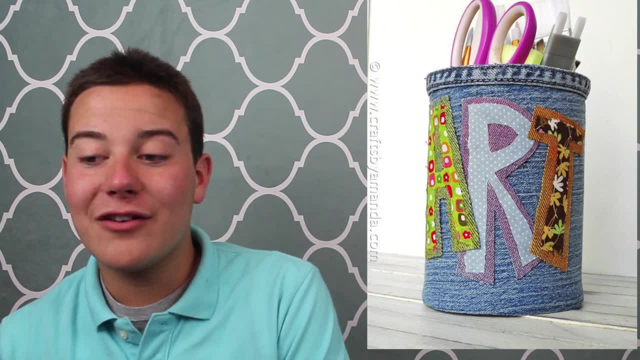 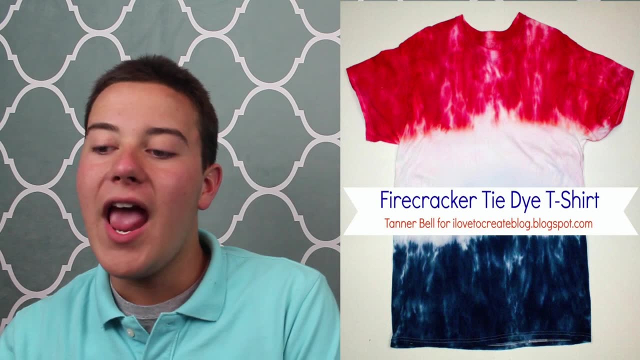 so I love this project for that. I actually created this Firecracker tie-dye design shirt for ilovetocreatecom and let me tell you, it is the best tie-dye shirt I think I've ever created and I am in love with it. 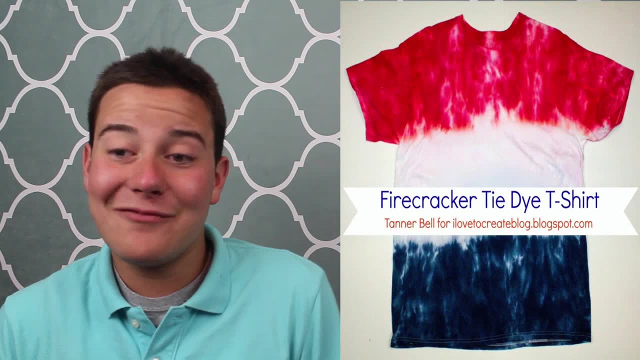 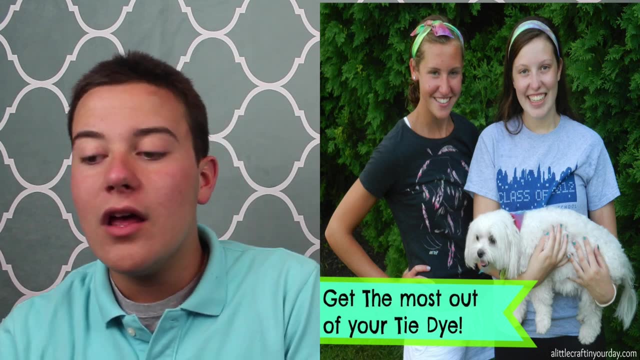 It is just a red, white and blue tie-dye design and really easy to do with the kids. Number seven was from my previous summer trip up to visit Courtney up in Pennsylvania. We tie-dyed a bandana and she shows how to get the most out of your tie-dye bandana. 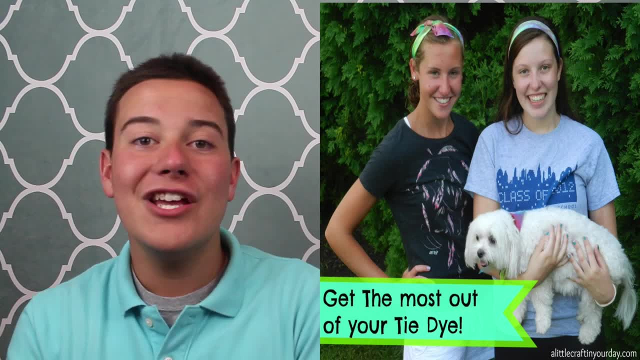 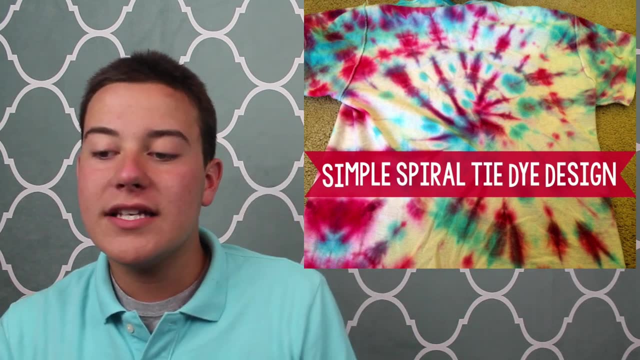 You can literally do so much with just one tie-dyed bandana. You're going to be amazed. Number eight is another video that I did right here on this YouTube channel, where I teach you how to make a simple spiral tie-dye design. 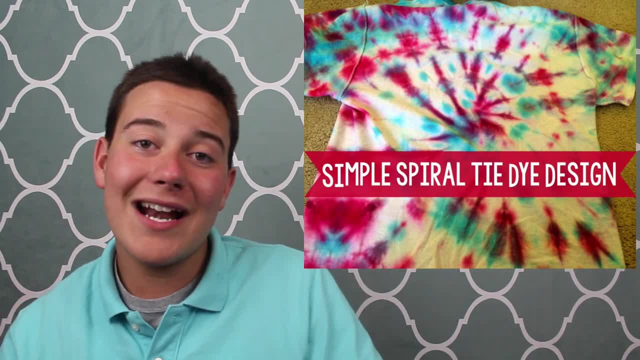 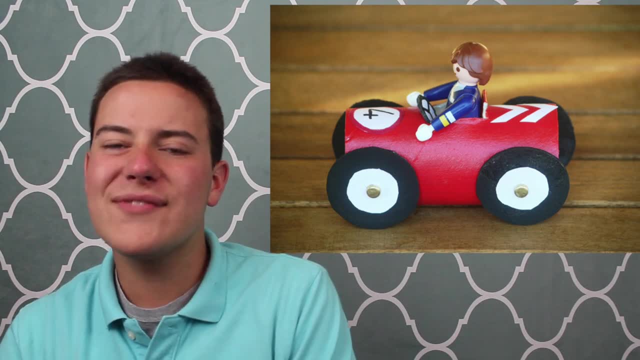 It is a really fun video and talks about a little bit about tie-dye and what you need to do to get the best tie-dye effects. Number nine is a toilet paper roll car. This one is fantastic because your kids can paint the toilet paper rolls and the toilet. 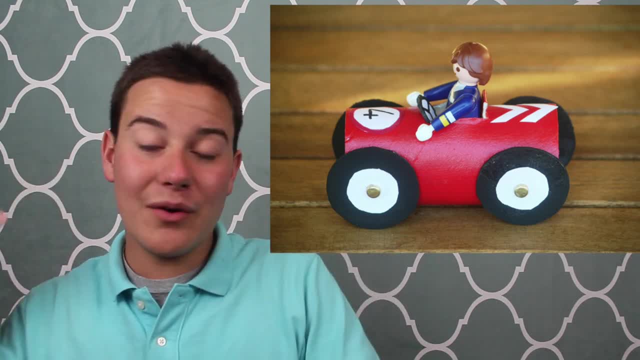 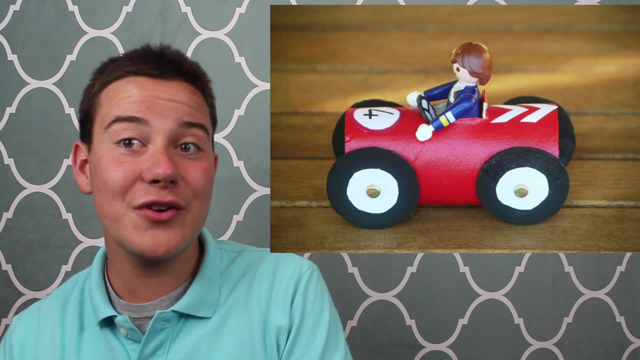 paper rolls are very upcycle friendly because you don't need to throw them away. I saved literally $1,000 for this. They're literally all mine to do crafts with it, and this would be a perfect craft, especially if you had a lot of friends over or anything like that. 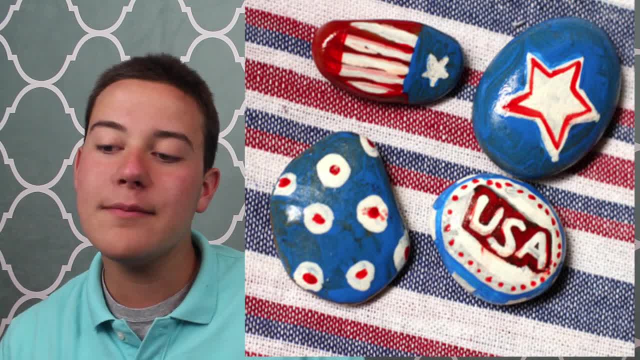 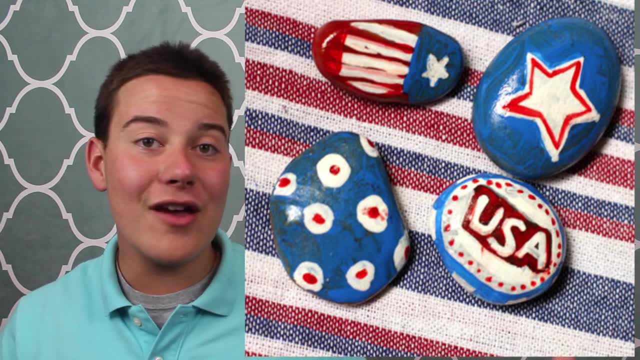 Number 10 is you can make patriotic tablecloth weights. Now, it doesn't have to be just weights for tablecloths, It could be paper weights, It could be a gift for the parent or anything like that, and you can just paint them whatever.